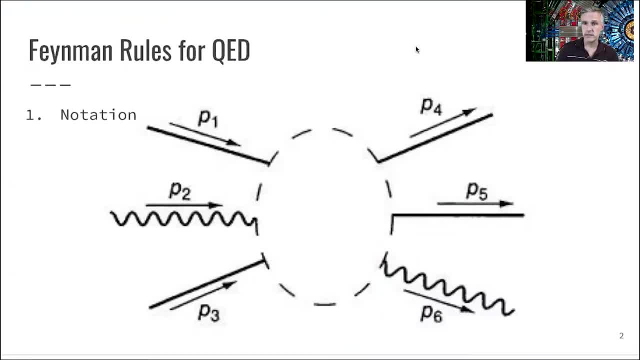 out. Okay, so the very first thing is to be very clear in our notation. So this is an arbitrary or generic QED Feynman diagram. We have only pointed out the incoming and the outgoing lines, So there is internal lines which I didn't mention here, Important to 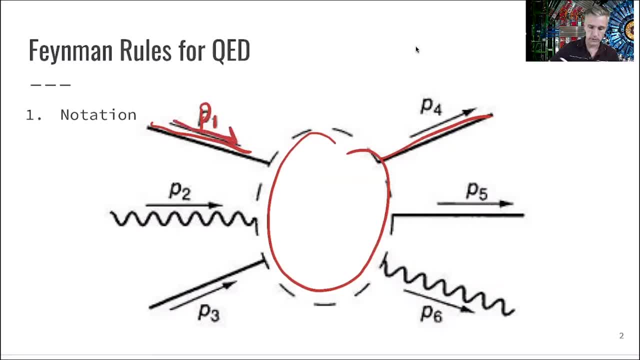 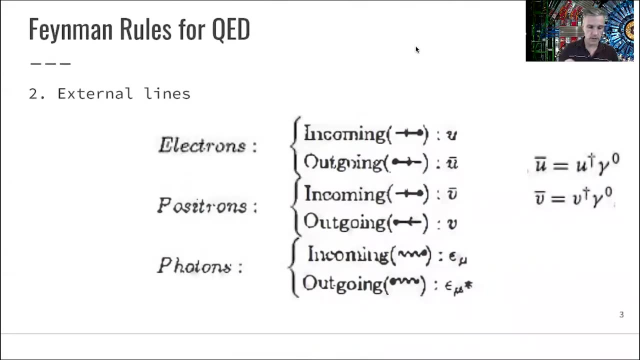 note the momentum and the directions. The directions are arbitrary. We just have to be clear on them and then treat them consistently. All right, so this is not different in our previous discussion. Then here comes the difference: Our external lines are either electron positrons. 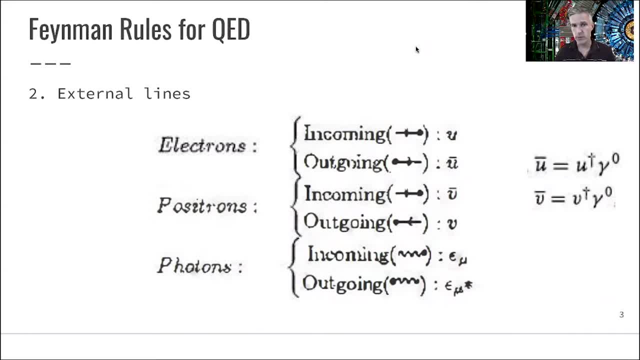 or photons, All right. So here we have fermions and photons, charged fermions and photons. So we discussed how the solutions look like our spinors U and V And for outgoing electrons, for outgoing particles, we have this adjunct vector here which is given by U, dagger, gamma zero And 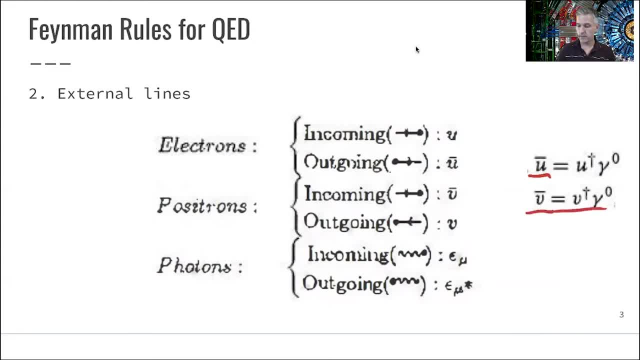 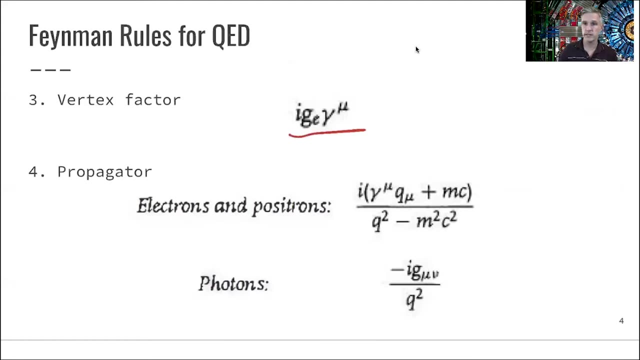 similarly for the incoming antiparticle: V dagger, gamma zero. For the photon, we have the polarization vectors For incoming and outgoing photons. All right, then we have a vertex factor Here. now, G 0 or GE is a constant and a dimensionless property, But we do have to have a gamma mu. 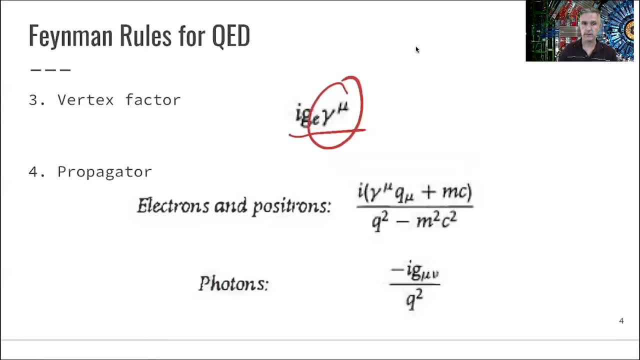 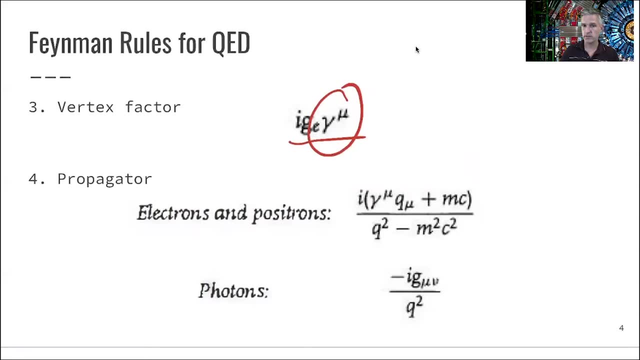 here, as part of our vertex factor For the propagator, our internal lines, we have a difference between electrons, positrons and photons, And that comes from the vector vector. So the propagator is responsible for the electrons, positrons and photons And that comes from the vector vector, vector And 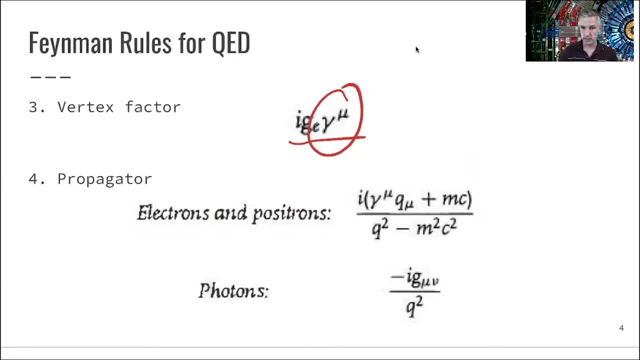 the fact that electrons are positive from the mass of particles. So we have vertex vectors which have this: 1 over q squared behavior, or 1 over q squared minus m squared behavior. So here you can already see that there's going to be a complication later when we evaluate or integrate. 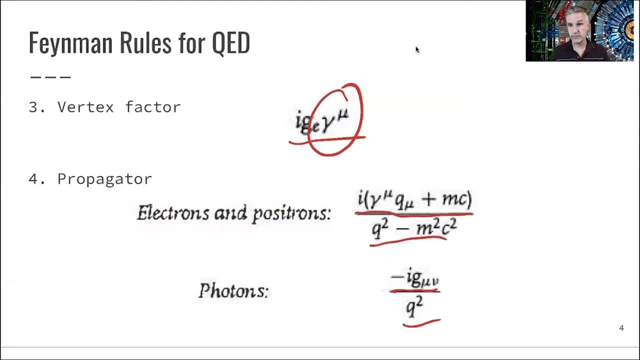 our momentum- Simply the same discussion I had before, and we already know how to solve this problem of infinities: by renormalizing, by having a cutoff and renormalizing- Excellent. So the next step, then, is very much the same. 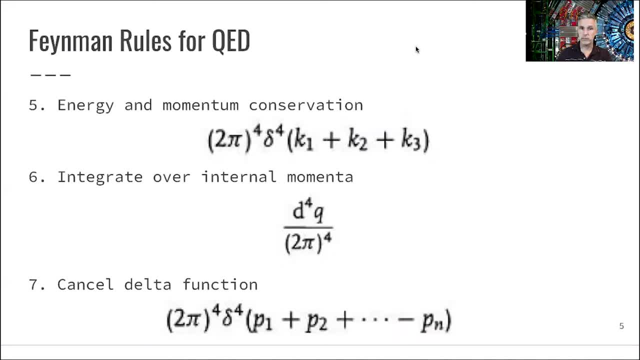 There's no change. We have to make sure that there's energy and momentum conservation and we enforce this. introducing delta functions, We have to integrate over each and every internal momenta and each internal line gets one of those integration factors And then, after we integrate, we have 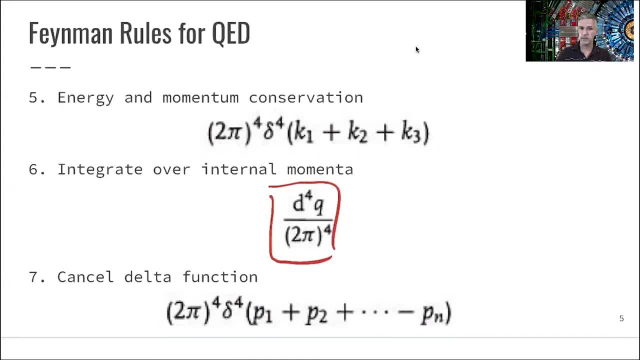 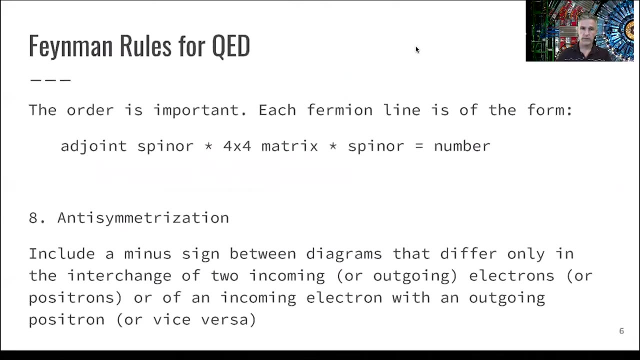 to. we are left with the delta function and we have to cancel that delta function. All right, In our toy experiment the order of things didn't matter. Everything we had in there was scalar numbers. right Here we do have a little bit more complicated problem. 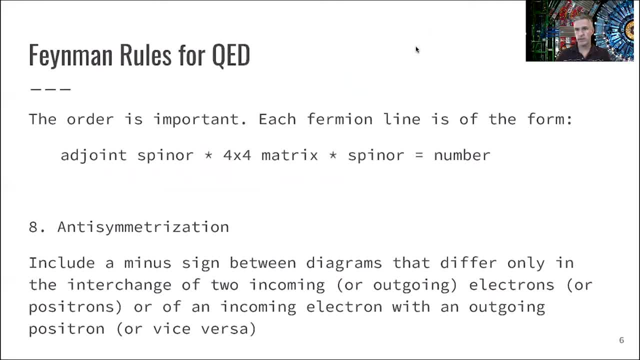 So there's an importance in the order of which we execute things. So what we want to do is form fermion lines, which is to follow a fermion as we go from the left to the right, And we will find things which are always of the form. 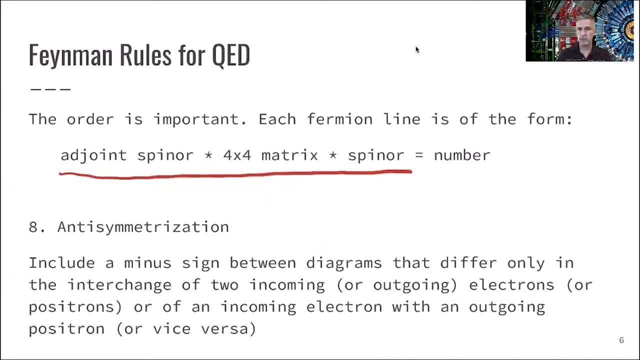 an adjoint spinor, a 4 times 4 matrix and a spinor, And the result of this is going to be a number All right, Great. There is one additional complication is accounting for duplications and making sure that the sign is. 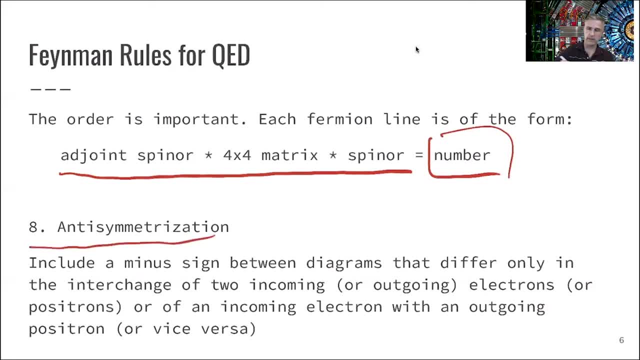 And I'm just mentioning this here. This will become more clear as we walk through examples. So there is an antisymmetration. There is an antisymmetration going on where we have to introduce a minus sign between the diagrams, between different diagrams that differ only. 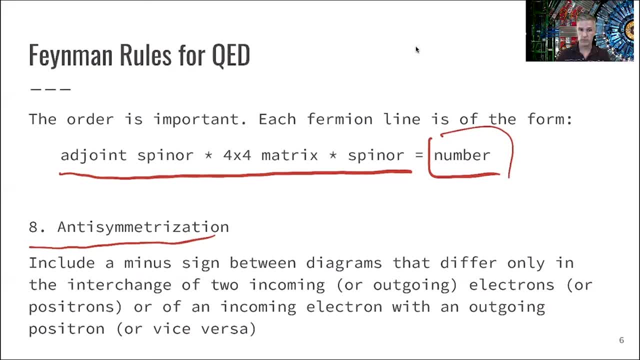 by the interchange or the exchange of two incoming or two outgoing electrons and positrons, and or the incoming electron with an outgoing positron. So if you have a diagram which is exactly the same but the two incoming electrons are interchanged, you have to add those two diagrams. 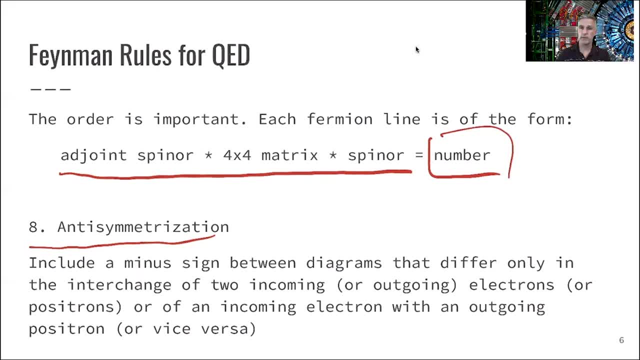 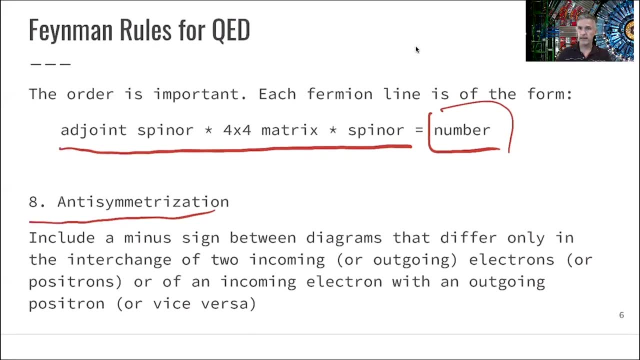 You have to add all matrix elements together before we calculate an amplitude. But you have to introduce a minus sign when you change those two particles. So with that we can now just basically calculate whatever QED process we want. All the tools are already here. 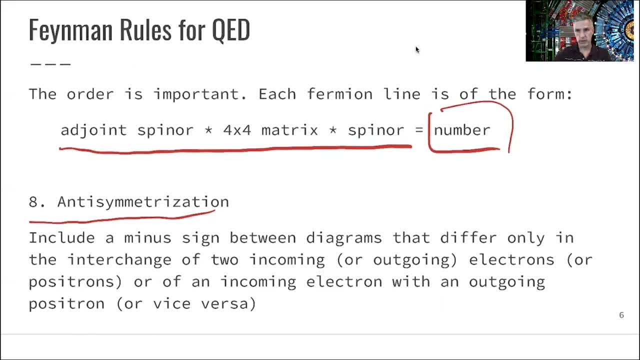 And what we want to do now, next in the next video and also in the recitation and homework, is to go through a few examples to get a little practice with this. There's a number of tricks which will become handy, and I'll 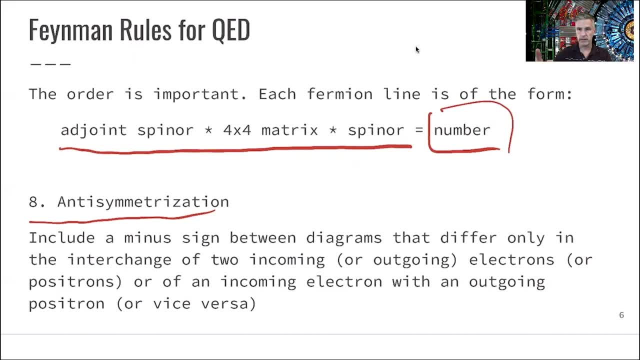 explain those. There are several videos. They're just mathematical tricks which allow us to quickly evaluate the multiplication of spinors and matrix elements and so on. All right, That's it for this video. Again, there is going to be another two or three videos. 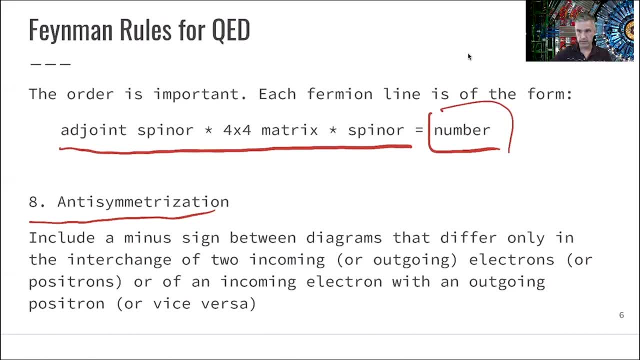 which deal with actually evaluating or calculating matrix elements. 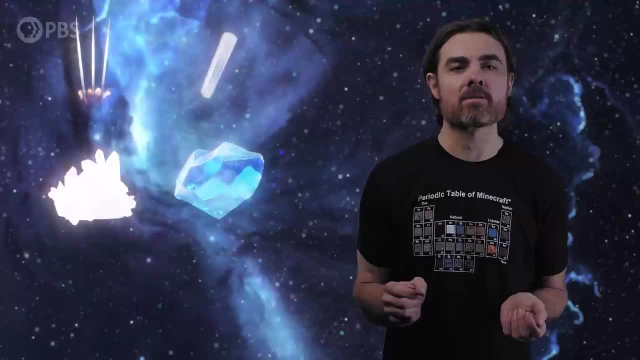 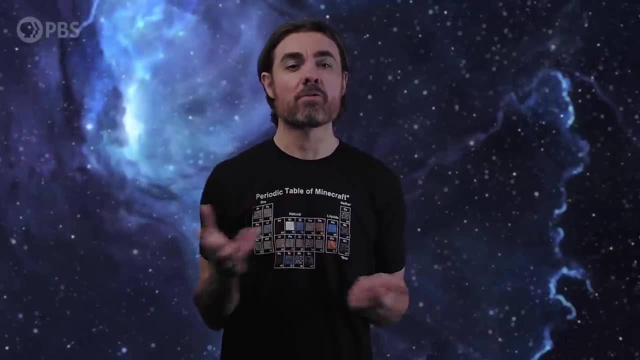 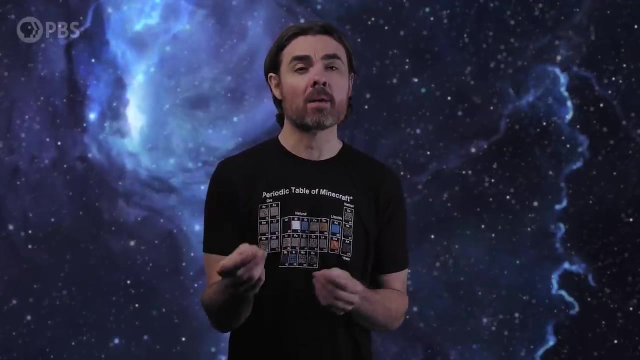 Adamantium, bolonium, dilithium, element zero, kryptonite, mithril, netherite, arachalcum and omtanium. We love the idea of fictional elements with miraculous properties that science has yet to discover, But is it really possible that new elements exist? 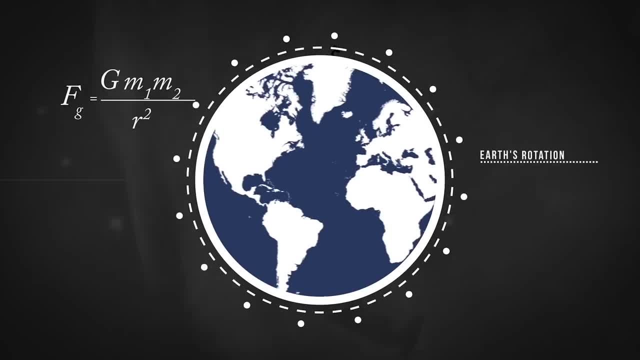 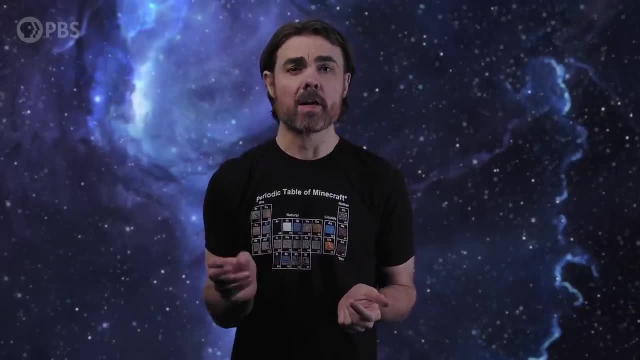 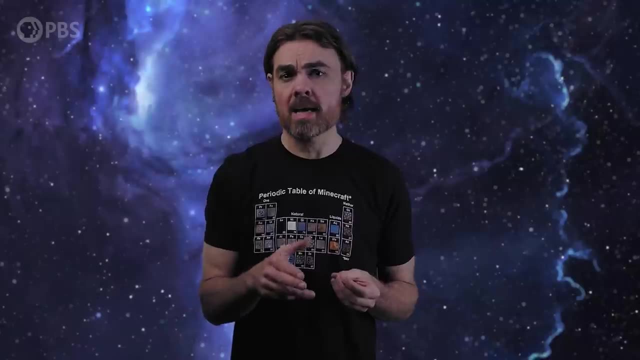 beyond the periodic table. Science fiction often imagines artificial or yet-to-be-discovered elements whose incredible properties will propel us to our star-faring future. But for anyone who's studied a bit of chemistry this may seem far-fetched. The elements of the periodic table are defined by the number. 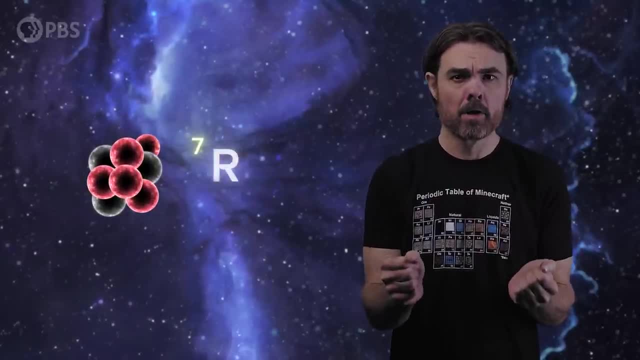 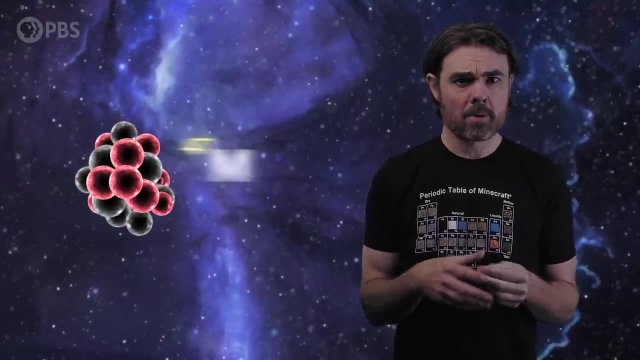 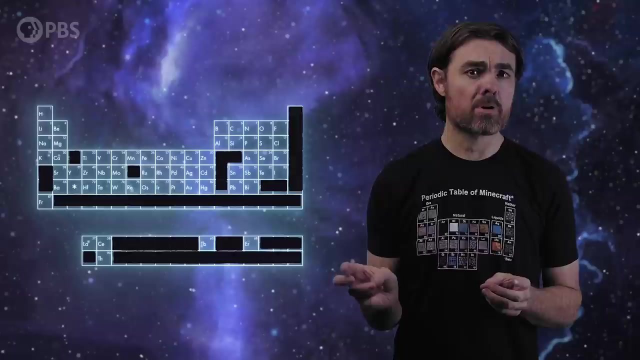 of protons in the atomic nucleus, the atomic number. So how can there be gaps for new elements? Sure, we could keep adding protons at the top end of the periodic table, but those seem to be hopelessly unstable and so hardly useful for building warp drives. But the fact is, gaps in the periodic table did exist: Atomic. 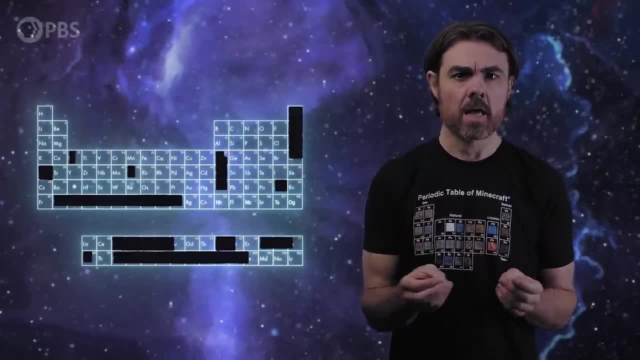 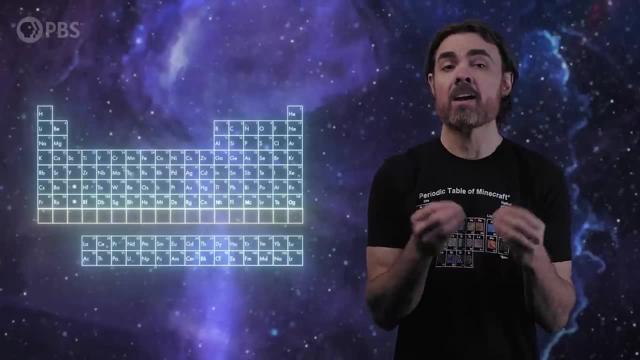 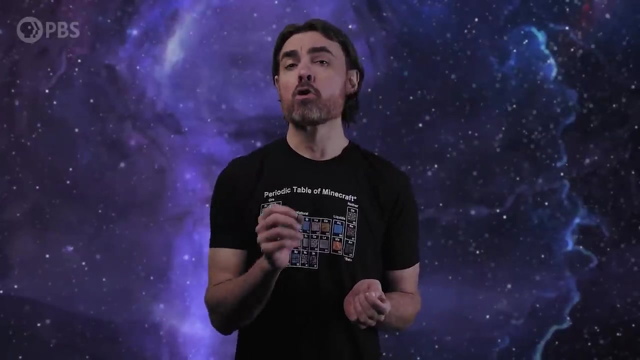 numbers that did not seem to appear naturally, And it may be that the current upper end of the periodic table is just another such gap beyond which there may exist an island of stability containing useful elements never before encountered. To understand the possibility of new artificial elements, we need to understand the possibility of new elements. 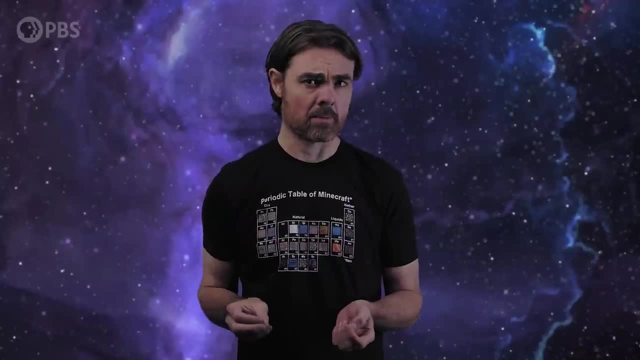 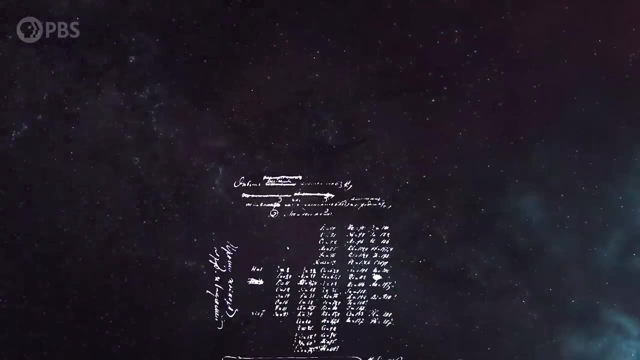 So let's start with the story of the first artificial element. We begin all the way back when Mendeleev figured out the periodic table. He arranged the known elements according to their atomic weight and noticed periodic recurrences of chemical properties as atomic weight increased.